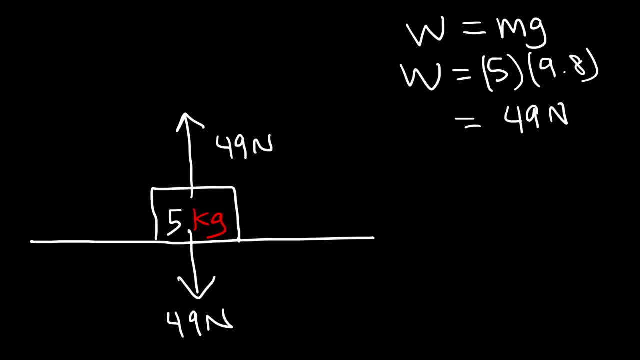 That force which is perpendicular to the surface, is known as the normal force. In this example it's an upward force. It's opposite to the weight force. Is there anything that we could do to either increase or decrease the normal force? 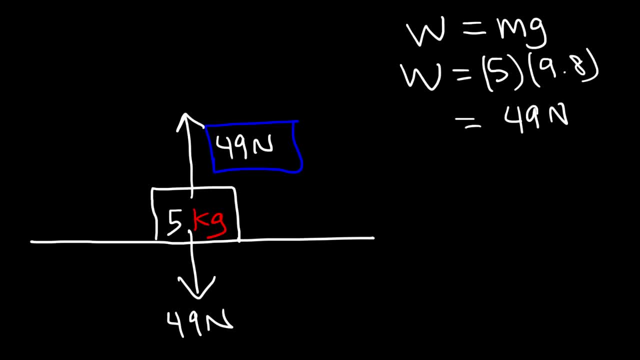 How can we do so without changing the mass of the object? The first thing you could do is you could press down on the object with another force. So let's say, if we apply a force of 30 N, So imagine taking your hand and pushing it down against the block. 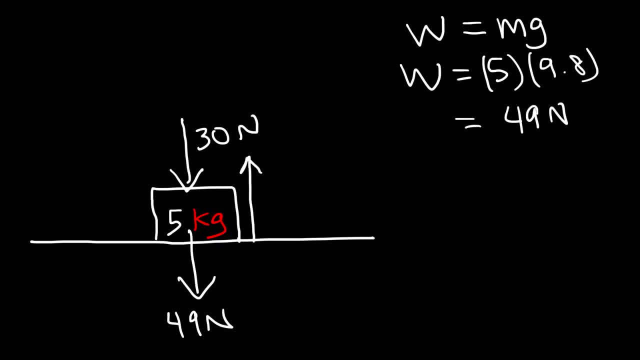 What force will this force exert? What will the surface exert on the block? What is the normal force now? Is it higher or is it lower than 49? If you exert a downward force on the block, the surface now has to exert a greater normal. 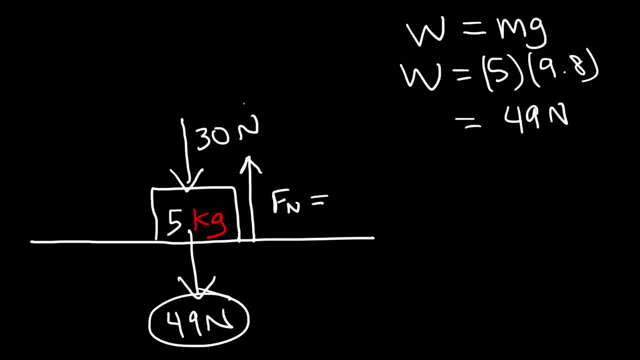 force. Not only must it support the weight of the block, but it must provide enough force to counteract that downward force that you're applying. So, therefore, any time you apply a downward force on this block, on an object, you increase the normal force. The normal force is going. 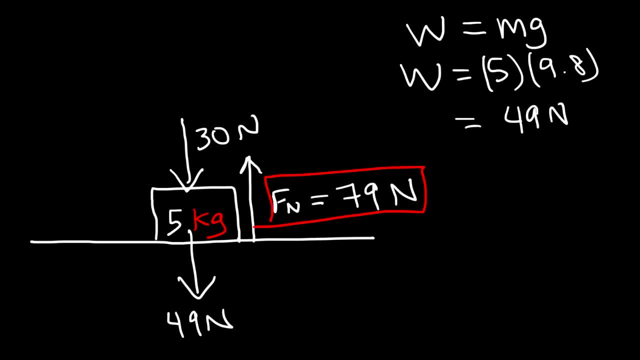 to be 79 newtons instead of 49.. So that's how you can increase the normal force- is by squeezing the block against the surface. Now, how can we decrease the normal force? What do you think we can do? One way to do that: 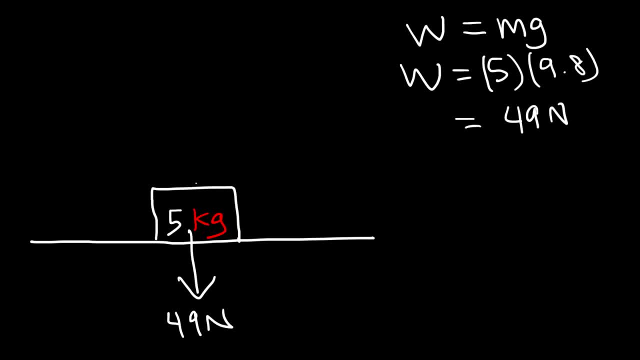 is to attach a rope to the block. Once you attach a rope to it, what you need to do is you need to pull up the block. You don't have to lift it off the surface, but if you apply an upward force acting through the rope, 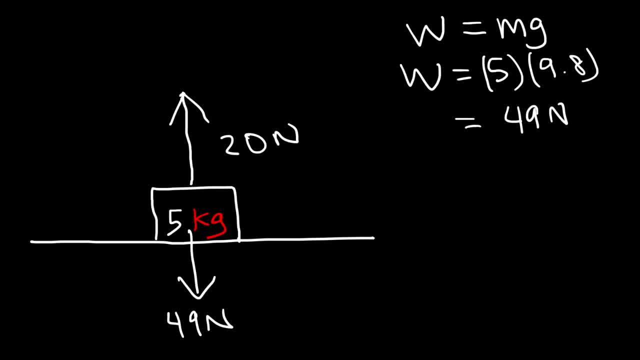 let's say, if we apply an upward force of 20 newtons, this block will feel lighter against the surface of whatever the block is on the horizontal surface. So now the surface doesn't have to support the entire weight of the block. It. 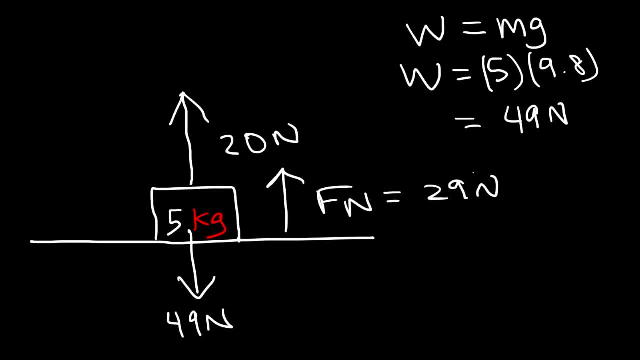 only needs to support 29 newtons because you're supporting 20 newtons out of the 45, out of the 49 newtons of the block. So when you lift up the the block, if you apply an upward force the surface, there's less pressure for the surface to 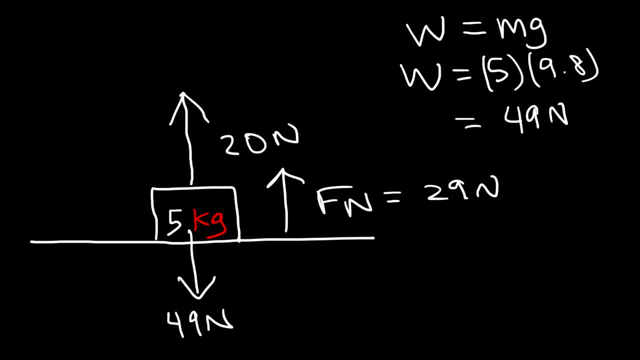 support the weight of the block So that decreases the normal force. if you lift it up, The total upward force- 20 plus 29, must add to the total downward force force in order for the forces to be balanced and for the five kilogram object to remain. 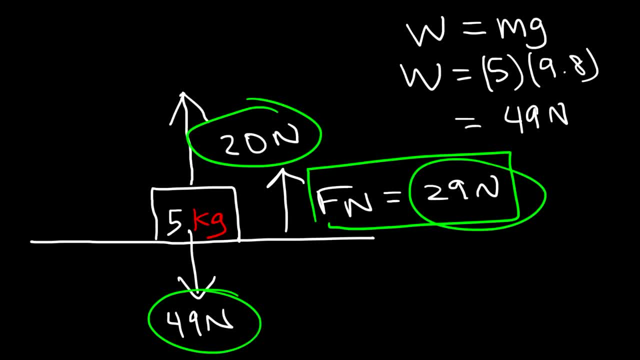 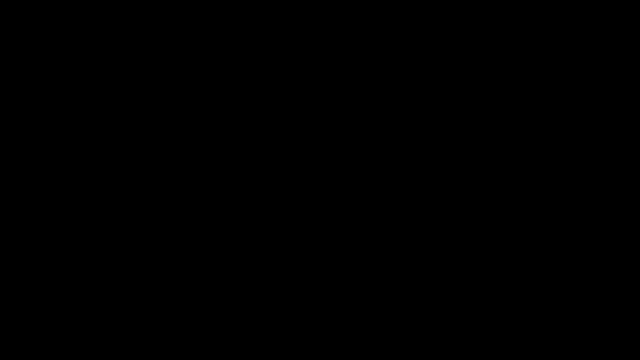 in equilibrium because it's currently at rest, And so anytime you try to lift up an object with a rope, the normal force will decrease. If you press it down against the surface, the normal force will increase. Now I'm assuming that, because you're watching this video, you're probably taking physics. 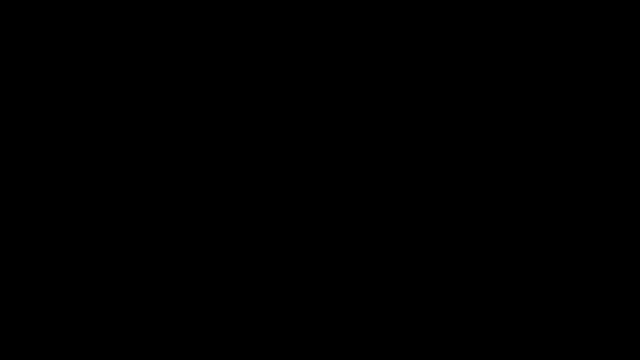 in high school or in college and it's important that you know how to set up a free body diagram and you know how to mathematically set up an equation to calculate different types of forces. But first I wanted you to understand the concept of normal force and when it's going to increase. 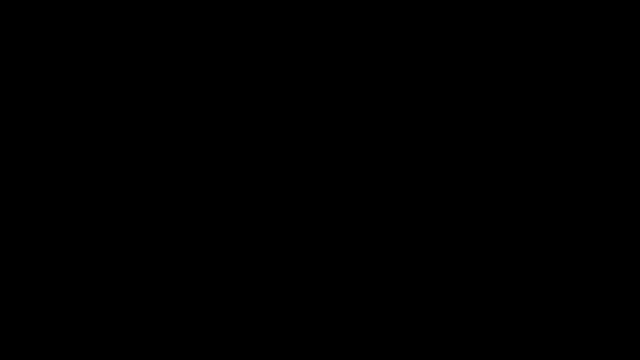 and when it will decrease. before I show you like a mathematical way of getting the answer, which is what we're going to do now. So let's say, if we have a 10 kilogram object and we wish to calculate the normal force, How can we set up an equation that will help us to calculate the normal force? if we just 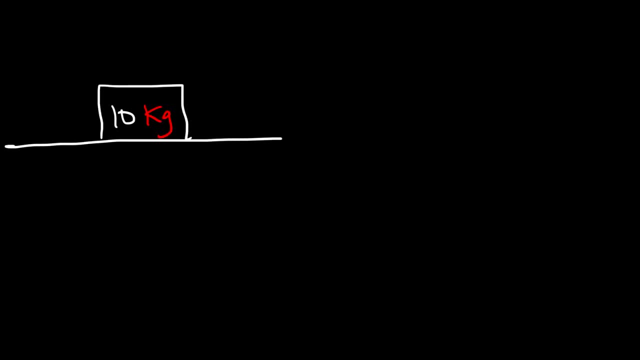 have this block at rest on this horizontal surface. The first thing you want to do is identify all these forces. in the y direction, We have a downward weight force and there's an upward normal force. So we're going to start with the downward weight force. 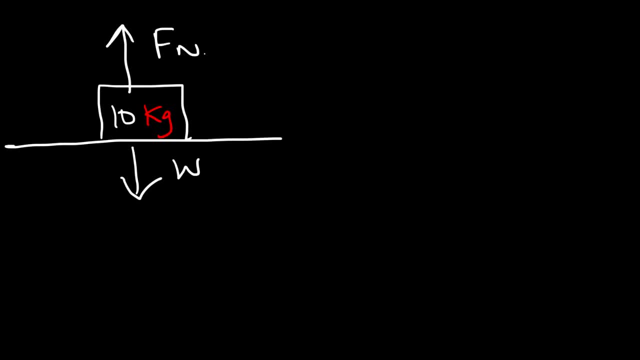 So we're going to start with the downward weight force. That's it. That's all the forces that we have in this example. So now we want to set up an expression that will give us the net force of the object in the y direction. 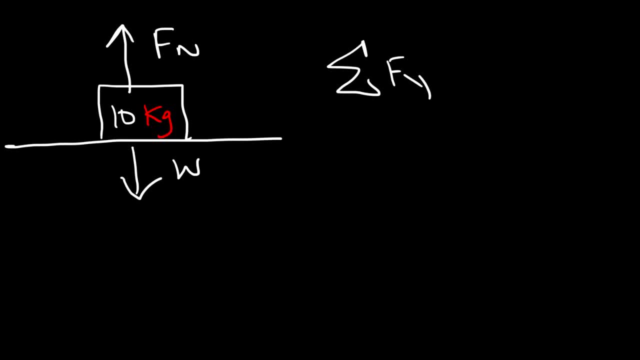 There's no forces in the x direction, so we don't have to worry about it. Now the normal force is in the positive y direction, So we're going to say it's positive Fn. The weight force is in the negative y direction. 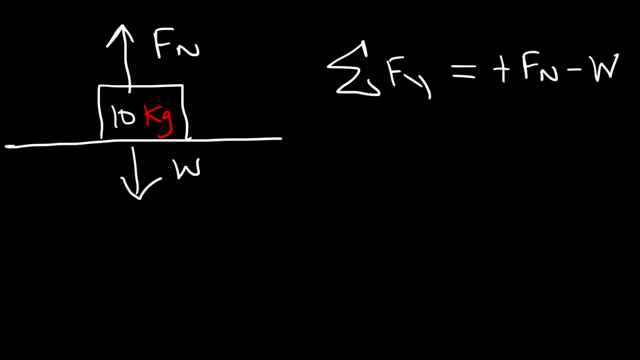 So we're going to say it's negative W. So we're going to say it's negative W. Our goal for doing this is to set up a process that's going to help us to calculate the normal force of this object, And understanding this process will help you to solve harder problems later throughout. 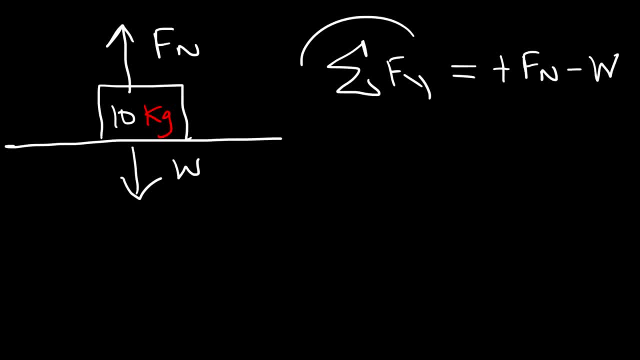 your physics course. So we need to know what to do with this, And you have to ask yourself: what is the object doing? Is it at rest, Is it moving with constant velocity Or is it accelerating? If the object is at rest or if it's moving with constant speed, the net force is zero. 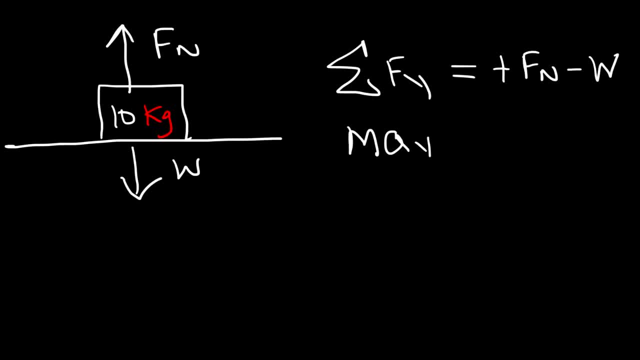 Now, if it's accelerating, you need to replace this with MA Newton's second law: net force is equal to mass times acceleration. But we know the block is sitting on the table or on the floor at rest. It's not accelerating upward or downward, it's simply at rest. 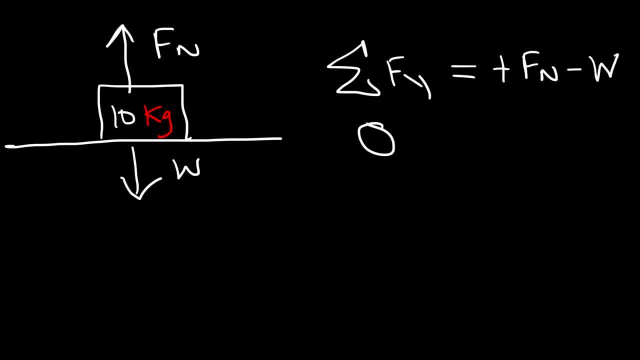 So, anytime it's at rest, and if it's remaining that way, replace the net force with zero. So now, if we add W to both sides, now we have an expression for the normal force. In this example, the normal force is simply equal to the weight, and the weight is mg. 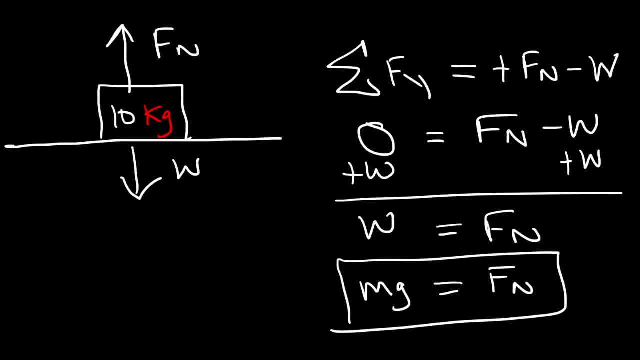 So if you have a flat object at rest on a horizontal surface, the normal force is equal to the weight force, as we've seen in an earlier example. So it's going to be 10 times 9.8, which is 98 Newtons. 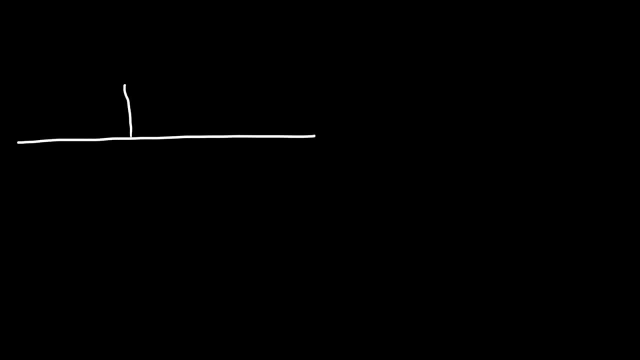 Here's the next example. So let's say, if we have a 15-kilogram mass resting on a horizontal surface, and this time we're going to apply a downward force of, let's say, 100 Newtons, Derive an expression for the normal force and then calculate the normal force with that. 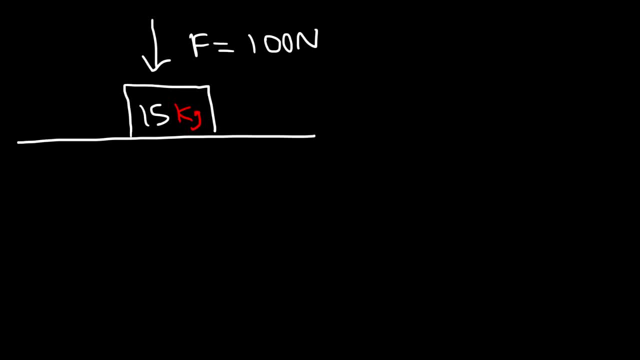 expression. So let's create a free body diagram. Let's identify a free body diagram. Let's identify all the forces that is acting on this block in the y-direction. So we have the downward weight force and there's an upward normal force. 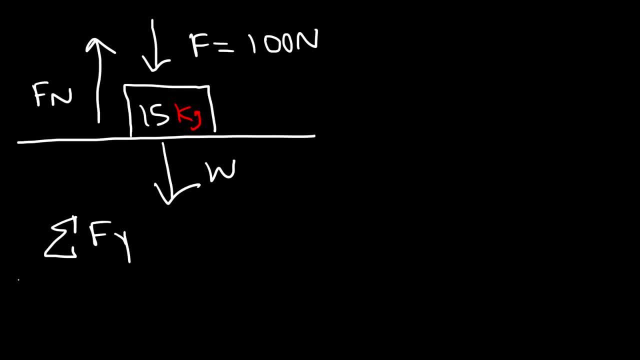 Now let's write an expression with the sum of all forces in the y-direction. So the normal force is going in the positive y-direction, The arrow is pointing up, So I'm just going to put positive Fn. Now the weight force is in the negative y-direction, so I'm going to put negative W. 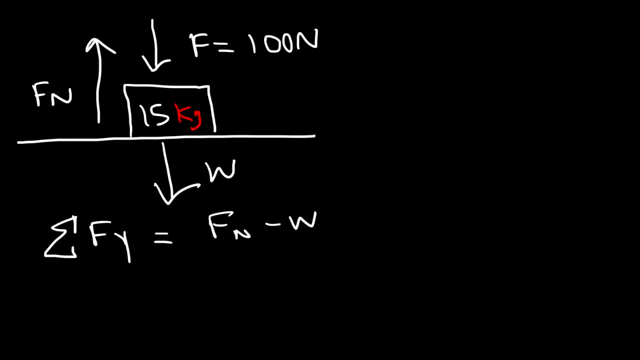 You don't have to put the positive if you don't want to, but in this case it's not necessary. Now this force is also in the negative y-direction, so I'm going to put minus F And because the block is at rest, it's not accelerating. Fy is equal to zero. 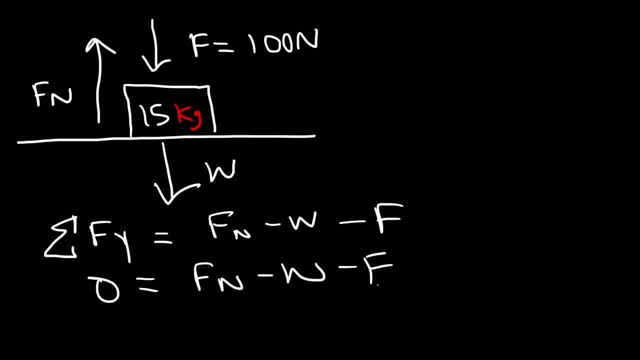 So we have this expression. Now what we're going to do is we're going to add W and F to both sides. So now all we have is the normal force on the right side. So the normal force, as we can see, is the sum of the weight force and the applied downward. 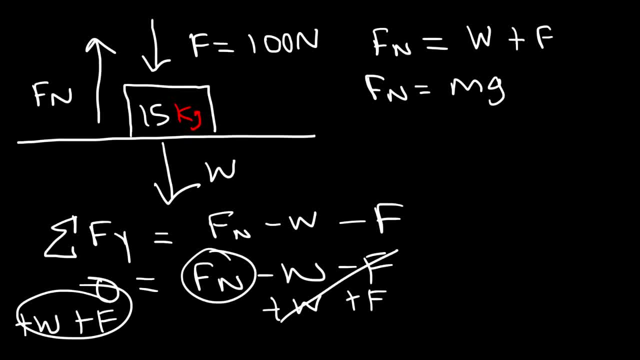 force. So it's going to be Mg plus F, So it's a mass of 15 times a gravitational acceleration of 9.8 plus the downward force of 100.. So now let me get my calculator And it's going to be 15 times the mass of the downward force. 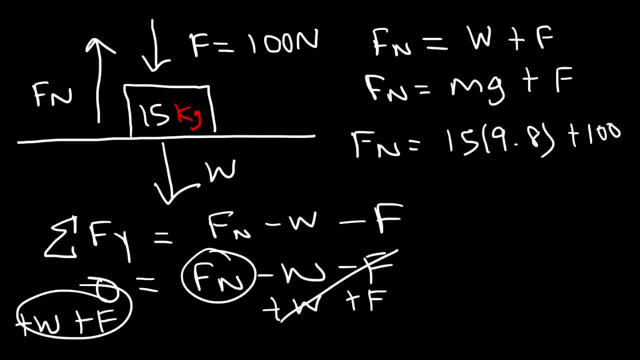 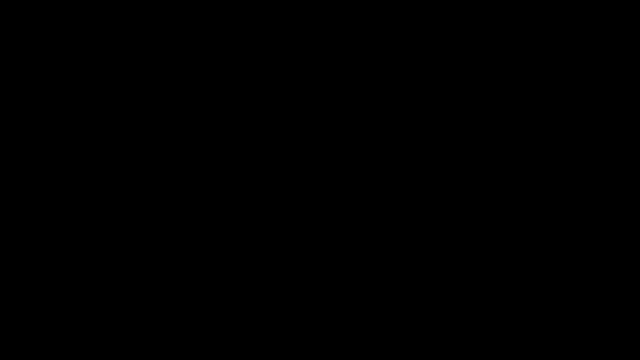 So 15 times 9.8, which is 147 plus 100. So in this example the normal force is 247 Newtons. So now let's look at our third example. So let's say, if we have a 20 kg mass, 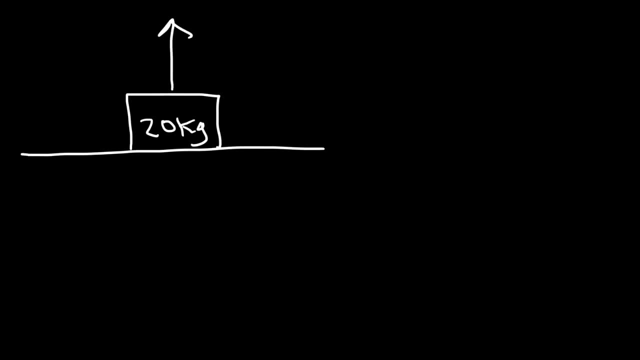 And this time we're going to apply an upward force. We're going to pull the object up- Okay, with a rope, and whenever you have a force that is acting through a rope, that force is known as the tension force. so I'm going to put T to represent the 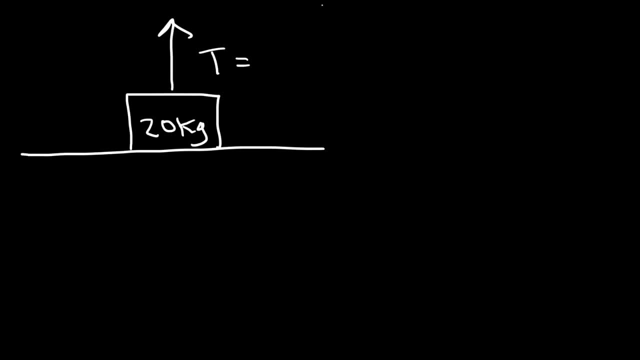 tension force. now, let's say the tension force is 100 Newtons in a positive Y direction. so then now we got to create the free body diagram. we have a downward weight force and an upward normal force. so, with this information, feel free to pause the video and write an expression that will help you to. 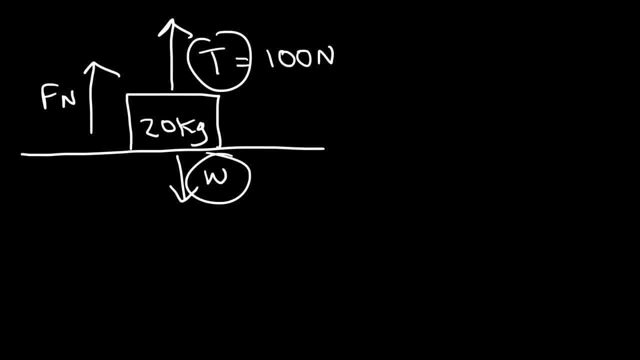 calculate the normal force using T and W. so let's write an expression with the sum of all forces in the Y direction. by the way, whenever you are lifting the object up, sometimes there may not be a normal force. if you get a negative answer, then what's going to happen? 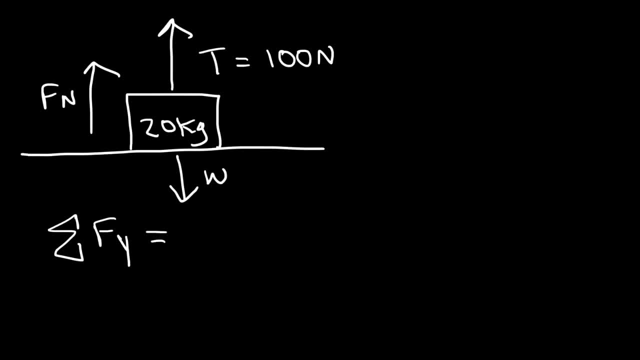 is, you're going to have to calculate the force and you're going to have to write an expression with the sum of all forces in the Y direction. by the way, remember that the tension force exceeds the weight force. if the tension force exceeds the weight force, the object is going to lift off the ground, and if it's, 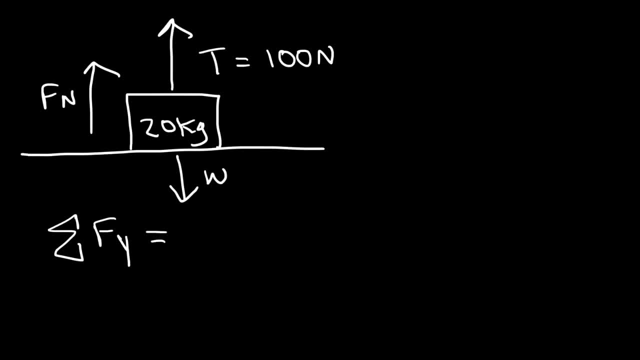 no longer in contact with the ground, there is no normal force. but let's finish this problem. so we have an upward normal force, we have an upward tension force, so this time it's going to be positive T or plus T, and we have a downward weight force. now we know that the tension force is going to be a. 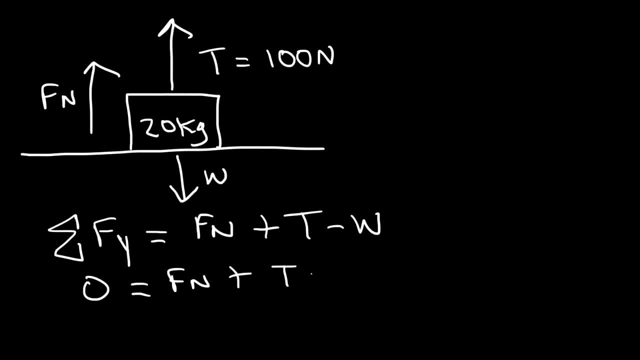 normal force. we know this is zero. so I'm going to add W to both sides and I'm going to subtract both sides by T. so the normal force is now equal to W minus T. so it's the difference between the weight force and the tension force. now 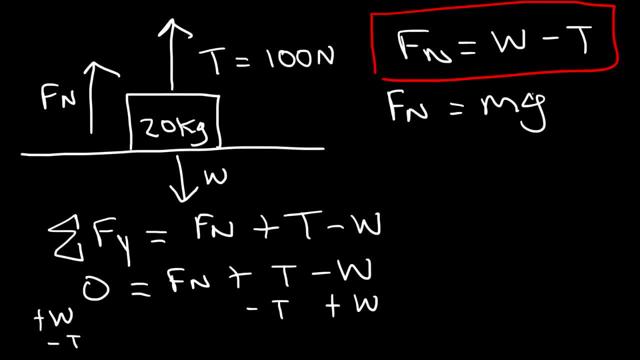 the weight force in this example is mg, as it always is, and that's going to be 20 times 9.8, which is 1.8.. and the tension is 100. now I want you to understand something: the tension in this example is less than the weight force, which means it's going to be a. 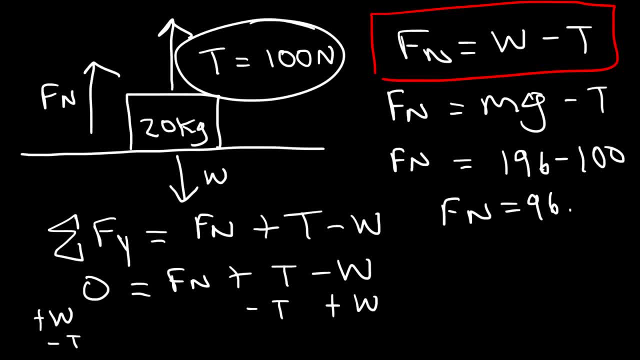 normal force, in this case of 96. but now let's say if the tension force, for example, was 300 newtons, if you use this formula, the normal force is going to be 196 minus 300 and you're going to get a negative answer, negative 104. so what's? 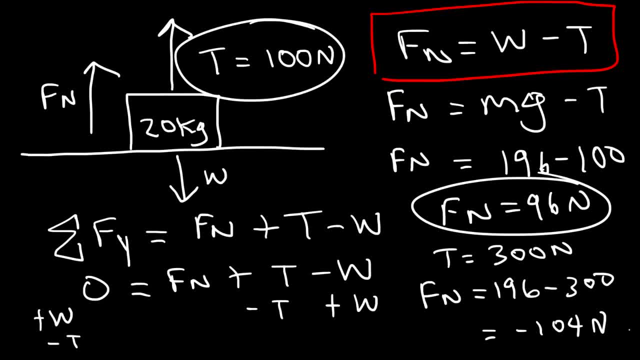 this means? if you see this, it means that the block is no longer in contact with the ground. it's actually being lifted up because the tension exceeds the weight force. so there is no normal force. so if you get a negative answer for the normal force, that means that there's none. it's no longer in contact. 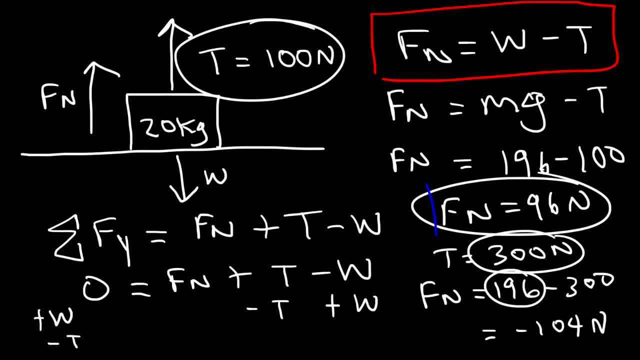 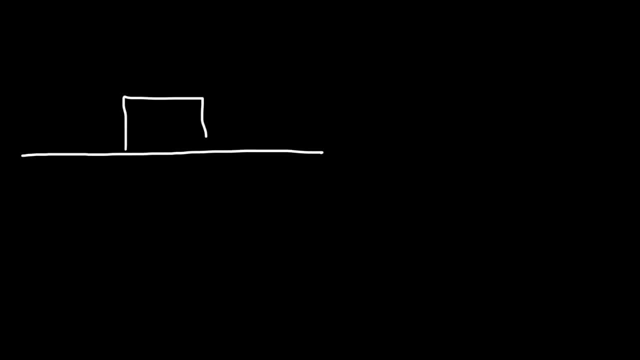 with the ground. so make sure you understand that. but for this example it's 96 newtons. now here's another interesting question. so let's say, if we have a 30 kilogram block and this time we're going to pull on a block with a 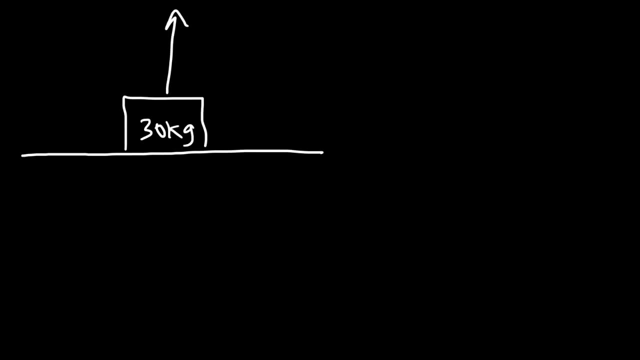 rope at an angle. instead of lifting it up directly, we're going to take a rope and pull it towards the right at an angle and let's say the tension force is, let's say, 300 units and the angle of this force is 30 degrees above the horizontal line. so with this information, go ahead and calculate the. 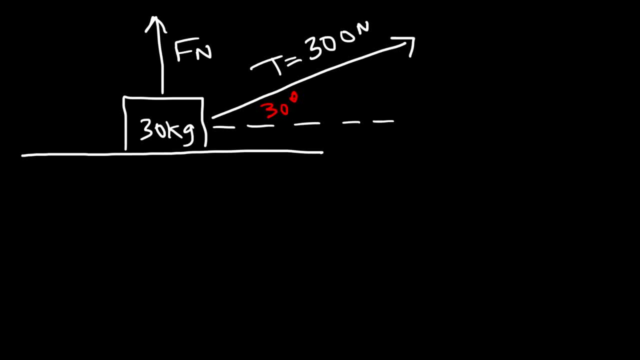 normal force that the ground exerts on the block. feel free to pause the video. so let's create a free body diagram. we've got a downward weight force, the upward normal force and the tension force at an angle. now you need to realize that because this force is at an angle, it has an X component and it has a Y. 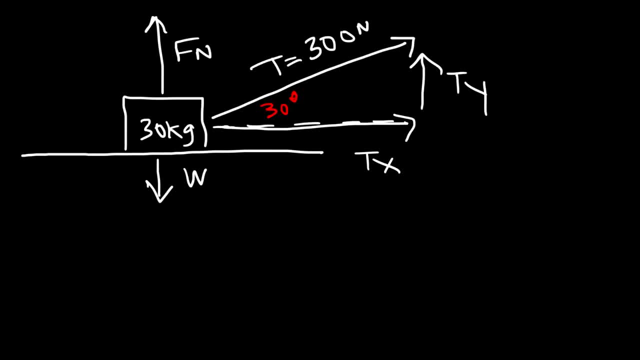 component, so we have T X and T Y now. the X component will give the block an acceleration towards the right if it exceeds the frictional force. but we're not concerned with T X though, because our goal is to calculate F, M, the normal force, and it's in the Y direction, so we 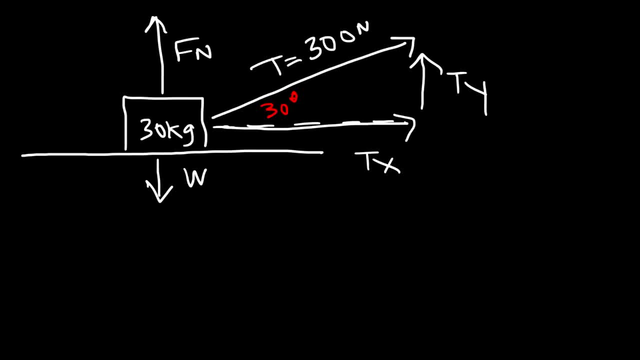 don't need T X, and a force in the X direction is independent with a force in the Y direction. at this instant, we need to focus on T Y, because T Y is the upward force in the Y direction that will decrease the normal force. so let's 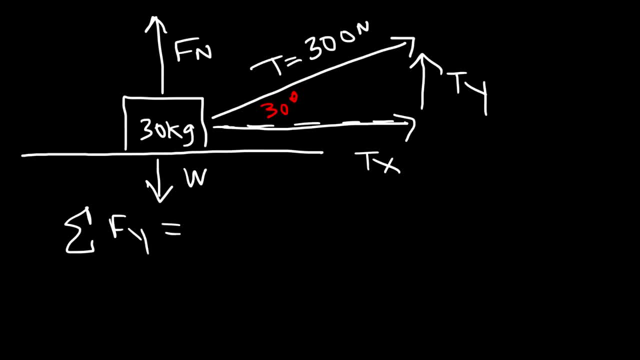 create an expression that will give us the sum of all forces in the Y direction, so it's going to be the upward normal force plus the upward T Y tension force. that's in the positive Y direction, and the weight force is in the negative Y direction, so it's going to be minus W. so now let's replace this with zero. we're 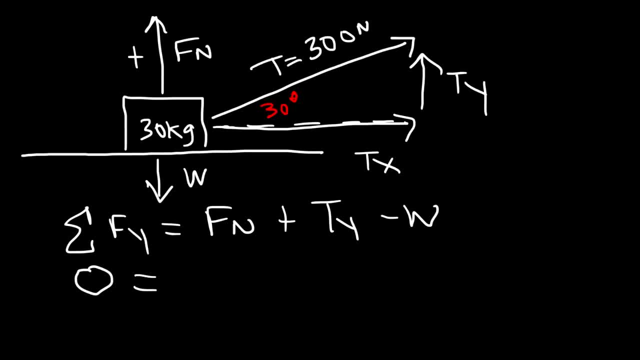 going to assume the object is at rest. if it's not, the normal force will be negative, so that means it's probably accelerating upward too. now let's add W to both sides and let's subtract both sides by T- Y, so we have negative T Y plus W is equal to F? M. 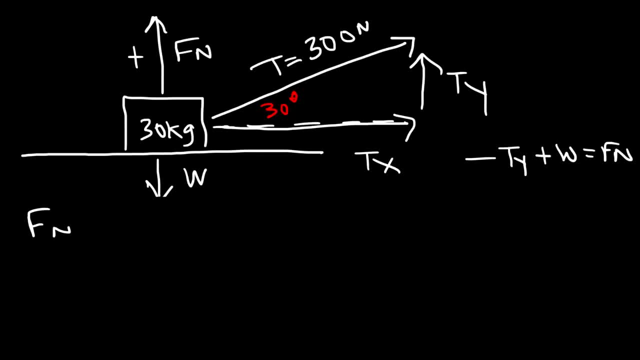 so we can rewrite that and say that the normal force is going to be the weight force minus the Y component of the tension force. now, what is the Y component of the tension force? it's important to know that T X is simply T cosine theta and T Y is T sine. 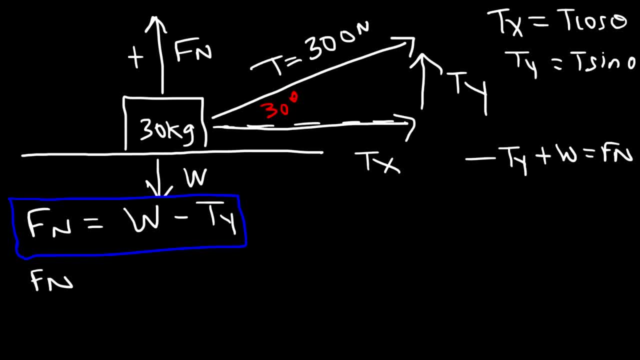 theta. so F N is equal to the weight force, which is M, G minus T Y, where T Y is T sine theta. so M is 30, G is 9.8, T is 300. and then times sine of 30, 30 times 9.8, that's 294 Newtons sine 30 is 1 half. make sure it's. 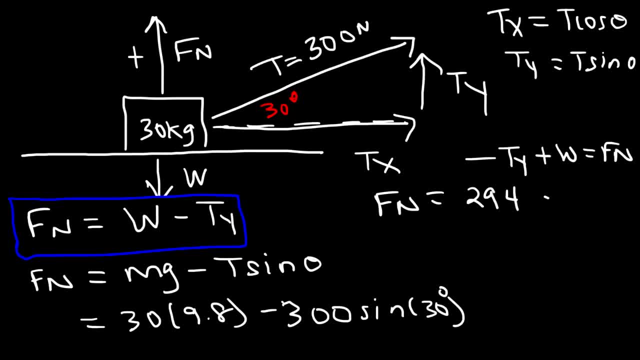 in degree mode, by the way, and 1 half of 300 is 150. so 294 minus 150 is 144. because we have a positive value for the normal force, that means that the block remains in contact with the surface. if we get a negative answer, that means that the tension force is strong enough to